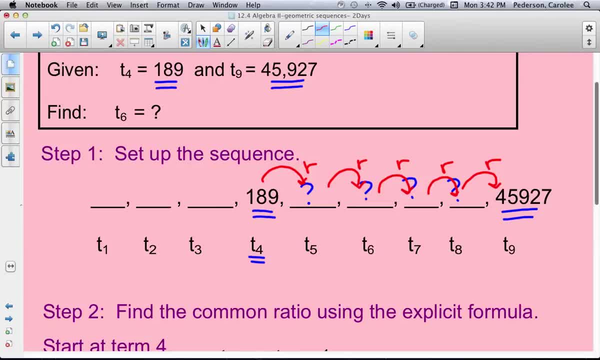 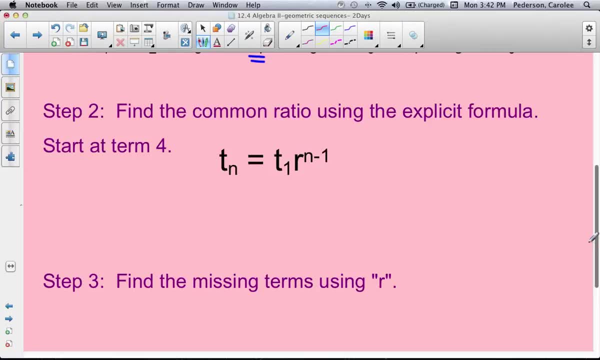 multiply it by five r's, So the r to the fifth power. So step two is to find the common ratio using the explicit formula. So to get to term four is where we're starting, And I want to finish at term nine. My common ratio is unknown. 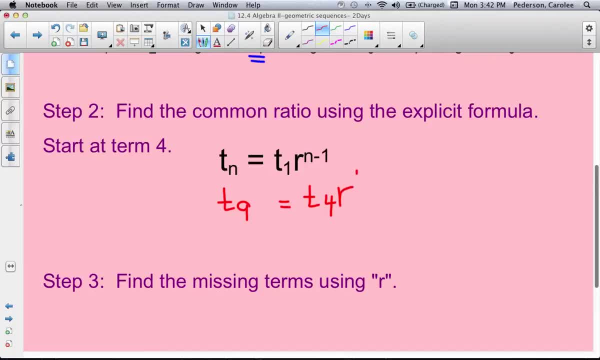 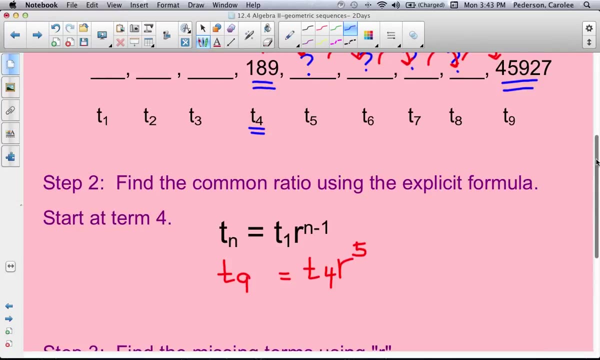 And I have five of those that I have to jump to, Five common ratios. Now let's substitute in the values we know, So we come back up here. Term nine was 45,927.. Term four was 189.. And then r to the. 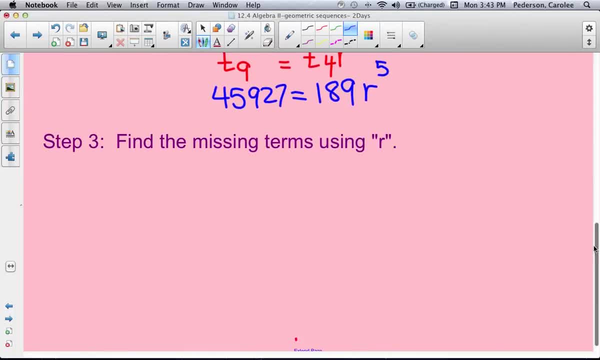 fifth power. Now what we're going to do is we're going to go ahead and solve this blue equation for r to find the common ratio. So step one is to divide both sides by 189.. Okay, Okay, Okay, Okay, Okay. 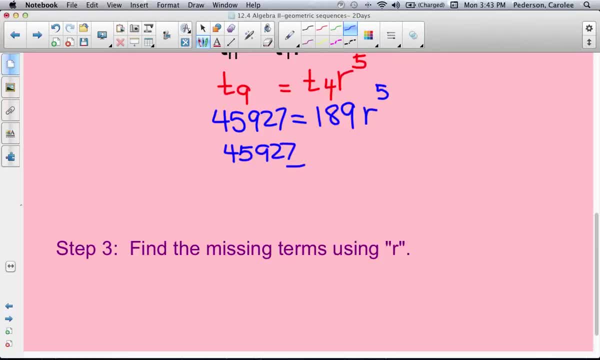 So 45,927 divided by 189.. And we get 243.. Now what we need to do is undo that fifth power, so we have to fifth root both sides. So R equals the fifth root of 243.. So in your calculator you go 5, math down to number 5, and then put in 243. 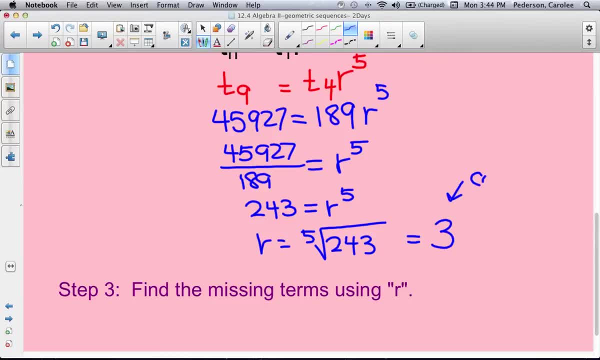 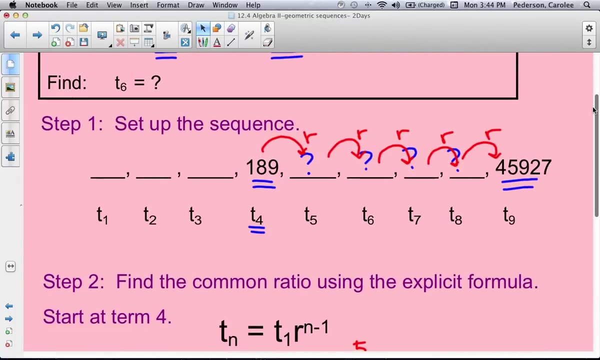 And you get R to be 3.. This is the common ratio. Now we can go ahead and use that common ratio to find other terms in the sequence. Alright, so let's answer the question now. I'm just going to erase these common R's. 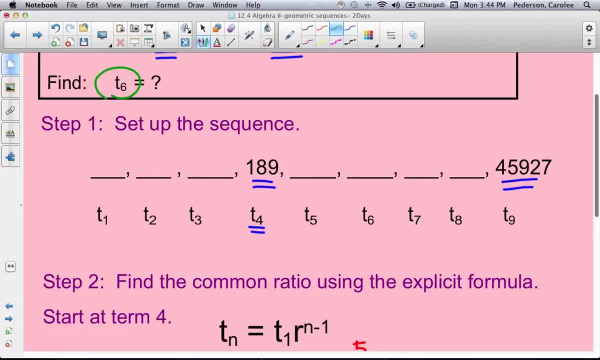 It asks us to find the sixth term. So I'm going to start with term 4, and I'm going to multiply it by 3.. So 189 times 3 is 567.. Now I'm going to take 567 and multiply it to 3.. 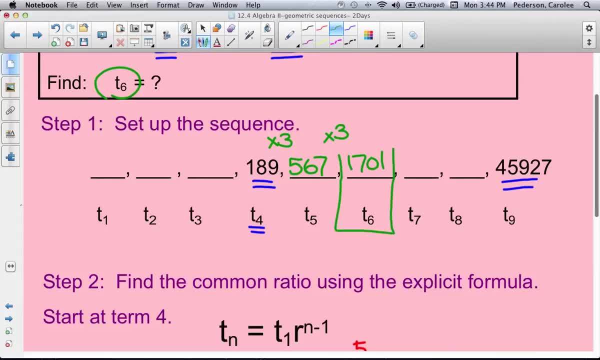 And I get 17.. Here is my answer for the sixth term, 1701.. 1701..